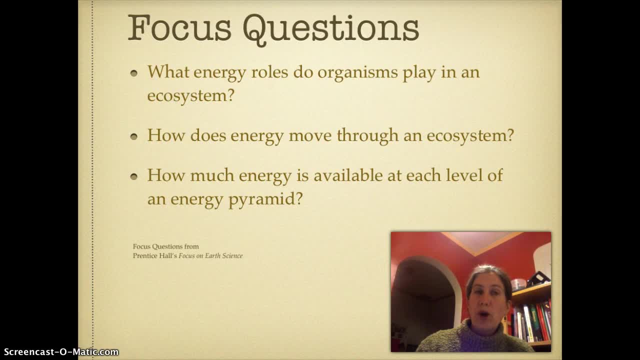 an energy pyramid. So you're going to need to stop probably the video, take some time to set up your Cornell notes Once again. on the right side you'll write kind of vocabulary and other things that you learned or other things that maybe you know. that would be helpful. 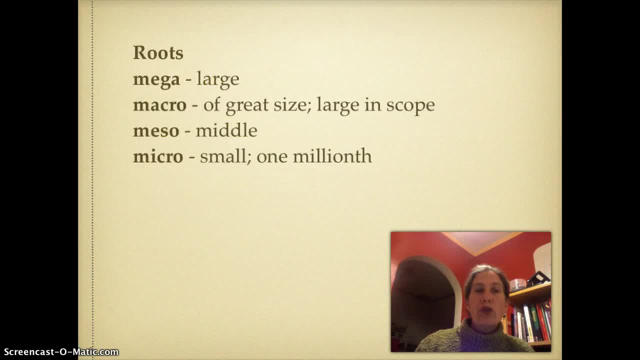 for you to understand these concepts. We also have a couple of root words that will kind of help us access the vocabulary Once again. in your science journal you're going to highlight these so that you know that we've studied them and you're responsible for them after this. So one mega is large macro of 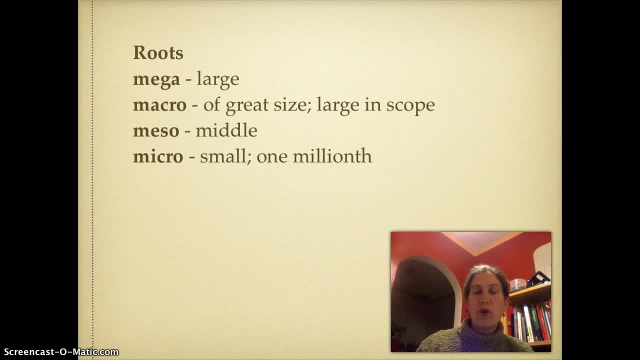 great size, large in scope, So we've talked about that before. macronutrients, the NPK that plants need in larger quantities, Meso, middle- and you guys have learned about Mesopotamia in your language arts class- And micro, small or, in particular, micro or micro or micro. 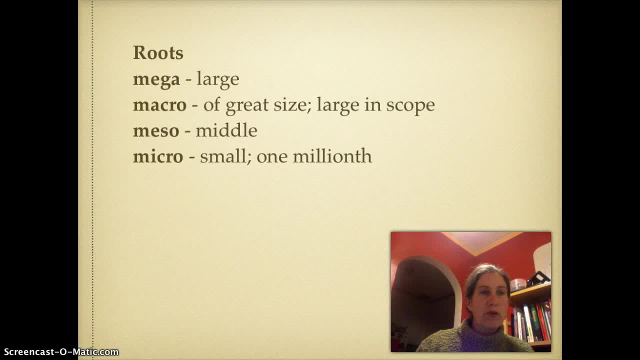 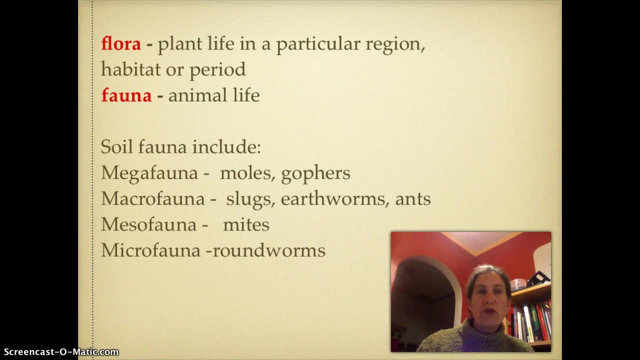 And micro large, and you guys have learned about micro or micro or micro or micro And micro large, and you guys have learned about micro or micro or micro. So two other really kind of helpful words to know are flora and fauna, So flora deals. 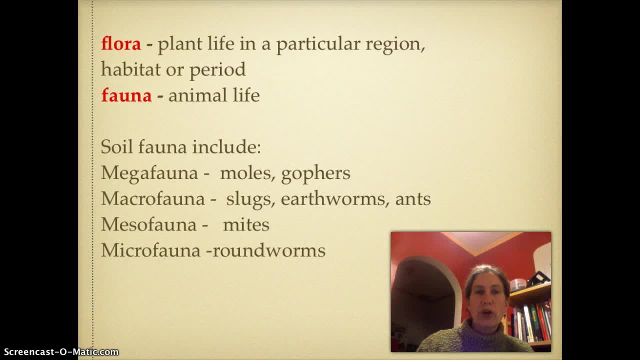 with the plant life in a particular region, habitat or geologic period, And fauna is the same, but that's the animal aspect. So, for example, when I lived in Fiji, I was really interested in learning about the flora of the tropical rainforest there. 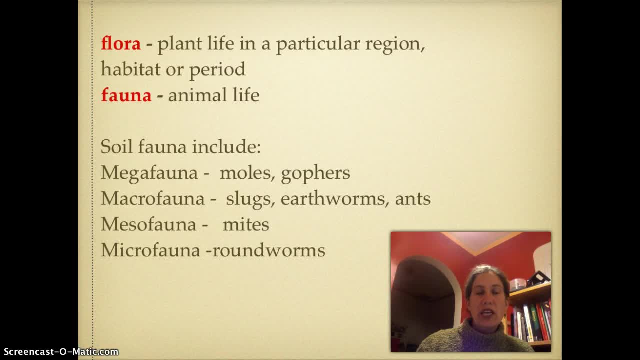 So, in particular, we're going to be looking and learning about some of the fauna in the garden. So we have our megafauna- unfortunately- gophers. We have some macrofauna- slugs, earthworms, ants- our mesafauna, mites, and then there's 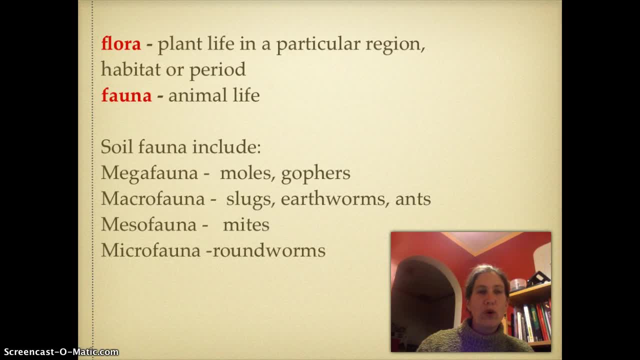 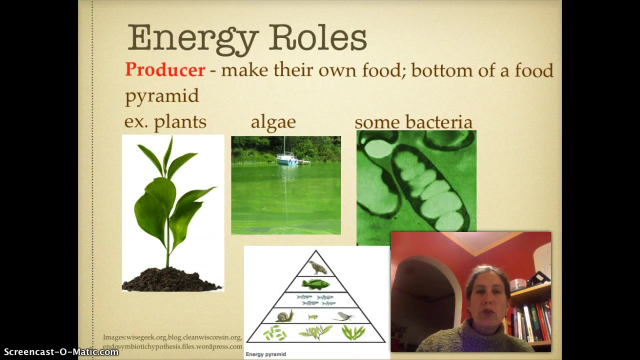 smaller things that you'd need a microscope to see, such as roundworms, And we will be looking at some of those under the special microscope equipment. Now, energy roles, So kind of. the three main ones are producers. They make their own food. 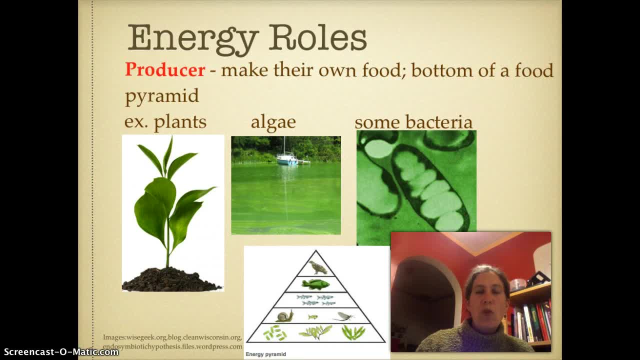 So, for example, plants, algae and some bacteria, When you look at a food pyramid such as the one on the bottom of the screen, this energy pyramid, the plants in particular are going to make up this large part of it, because everything else is they're getting their energy, which was produced from sunlight. 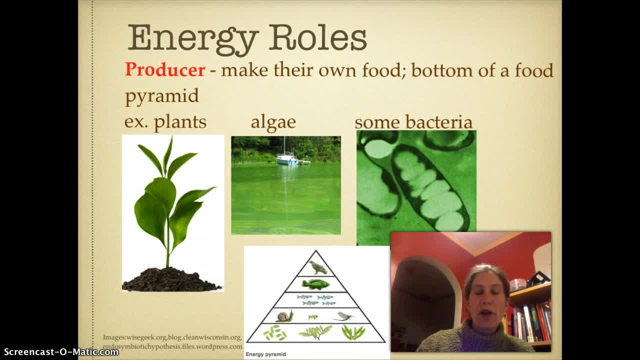 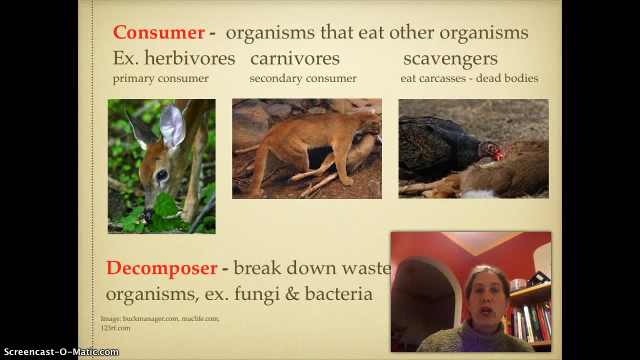 So from that bottom, the bottom, energy level, Consumers. So consumers are organisms that eat other organisms. So, for example, herbivores, also sometimes referred to as primary consumers. primary because they're eating the plants. Carnivores, which are meat eaters, are sometimes referred to as secondary consumers because 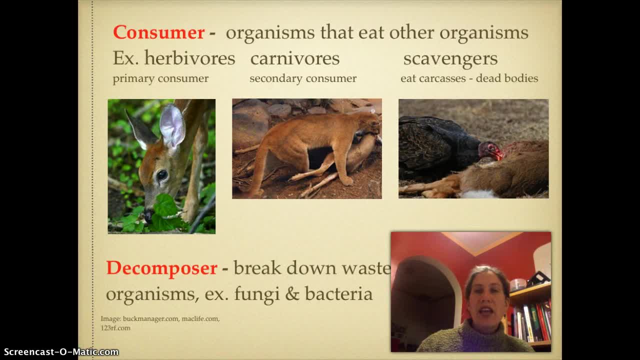 they are eating the primary consumers, And then scavengers. they eat carcasses, such as turkey vultures, and a carcass just means like a dead body. And then we also have the decomposers. Those are things that break down the waste and dead organisms, for example fungi and 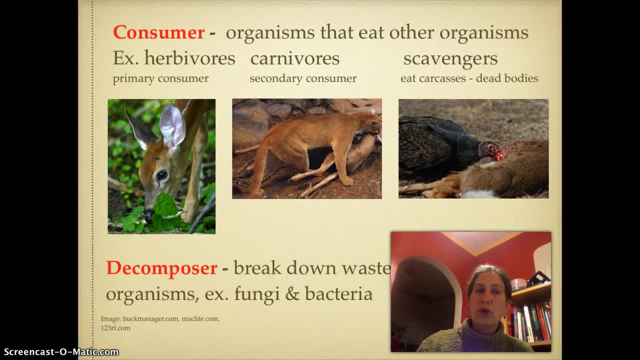 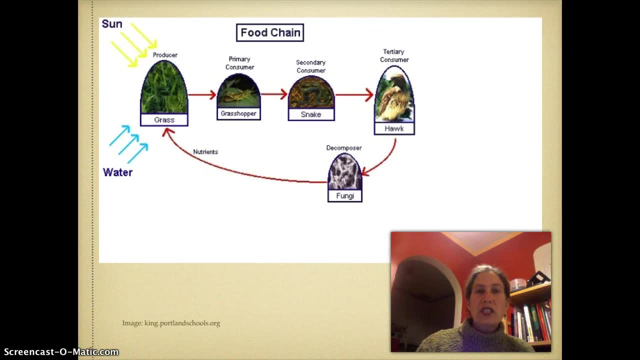 bacteria. Once again, you need to be stopping the notes. I'm sorry, stopping the video periodically and taking notes, So here's just a simple. Okay, Here's an example of a food chain. So once again you have your producers, your grass that's being eaten by a grasshopper. 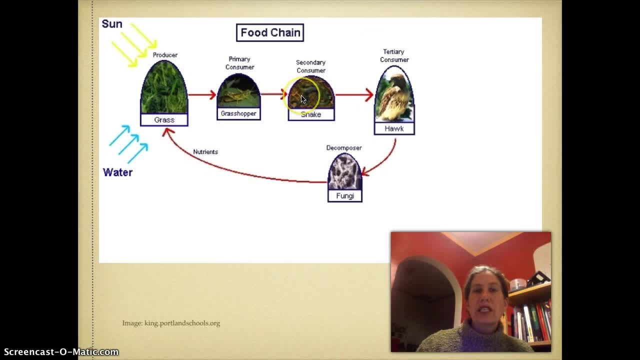 a primary consumer. That grasshopper is eaten by a snake And then the snake is eaten by a hawk, So that's a tertiary consumer, typically because energy is lost every single time. It's about one tenth or about 10%. It's what's able to be taken in in terms of the energy at each level. 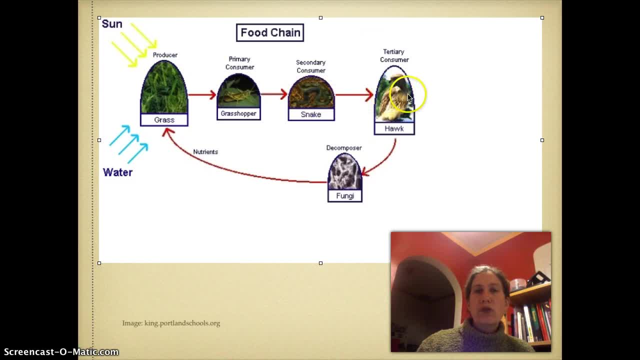 So it's a huge loss: 90% loss at each level. Most food chains can't really support anything above a fifth level consumer. And then you have the decomposers, the fungi. you know that would eat the hawk when it. 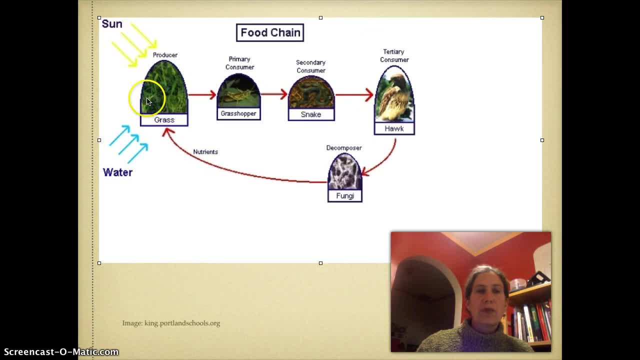 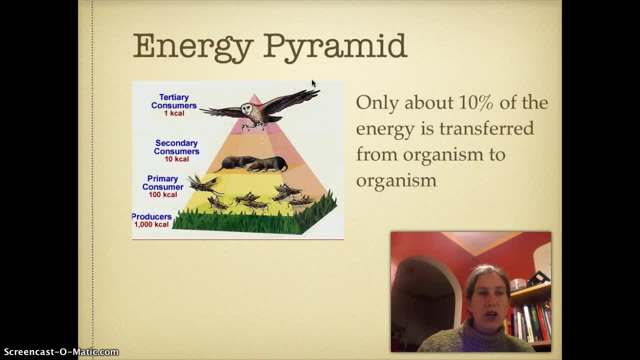 dies and it would go back into supporting the grass being grown. So here's a picture of an energy pyramid. You saw it earlier on the slide on producers. So once again you see that the producers have this huge area down on the bottom. 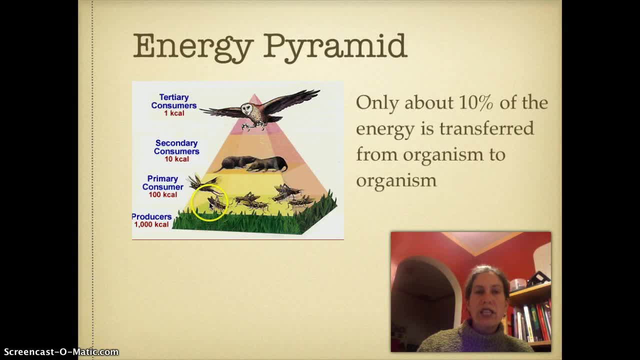 And the grasshoppers that eat them. you know only get one tenth or 10% of the energy from that. So you know, by the time you know it gets all the way up to the owl at the top level. 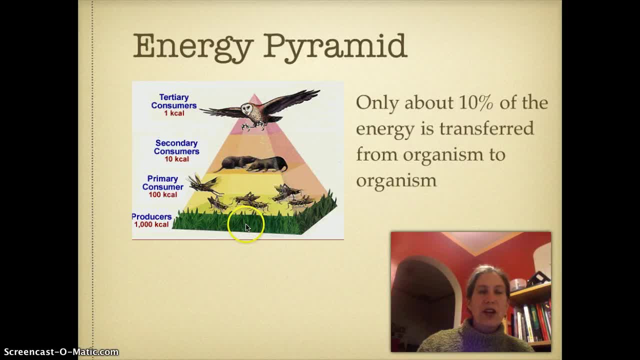 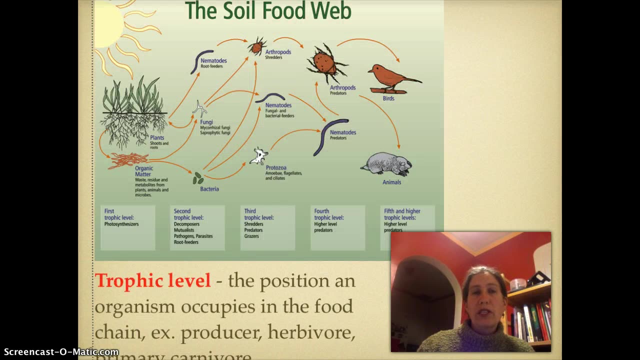 this tertiary consumer. for every thousand you know kilocalories of grass that were eaten, The tertiary consumer is only getting one kilocal of that energy. So let's look at the soil food web, because that's what we're going to be particularly 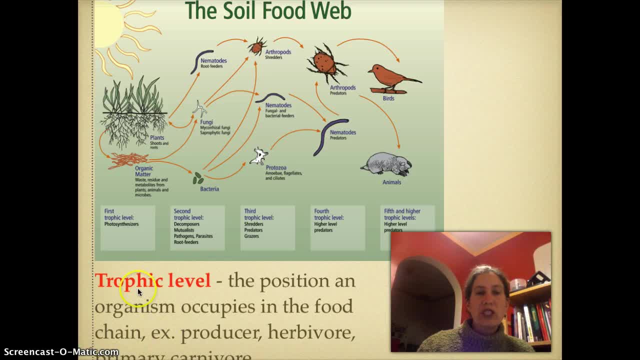 concerned with- And here there's a new vocabulary word, which is trophic level, and that's the position an organism occupies in the food chain. So we talked about already kind of the plants that photosynthesize. those are on the first. 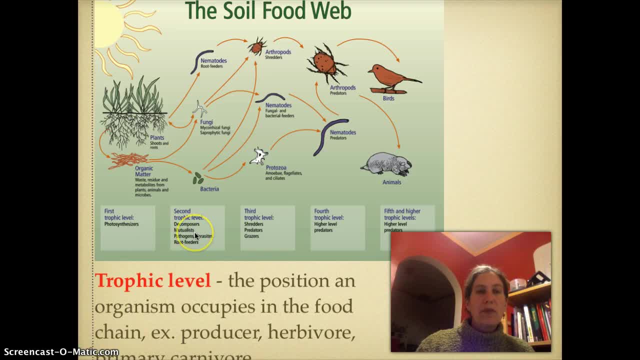 trophic level. Okay, And then we'll get into some of these other more specific words like mutualist and pathogens later. So you can kind of see it's a pretty complex. so it's a little bit different than a food chain which is just one thing after the other. 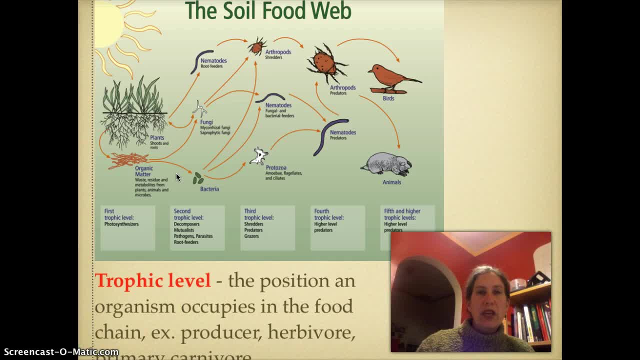 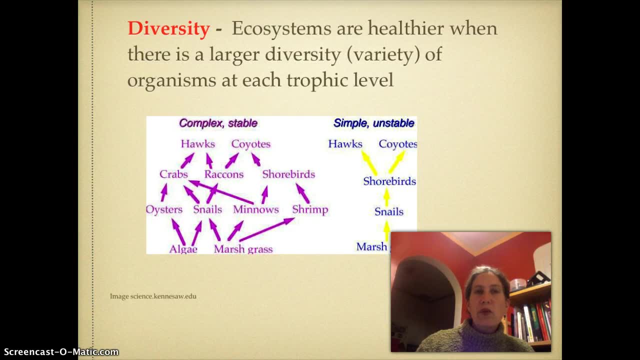 But this shows all the interrelations in, you know, in the environment, And the thing that I really want to point out is diversity. So ecosystems are a lot healthier when there's a lot more diversity. and we're going to play that game. So I'm going to show you a little bit of an example of that, and then I'm going to show you a little bit of a picture, And then I'm going to show you a little bit of an example of what we can do to kind of 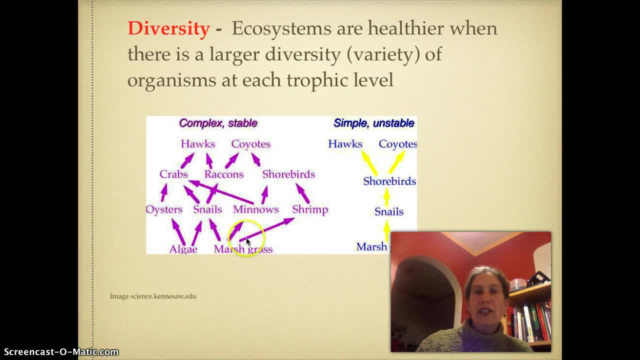 just show the interconnectedness. So when you have a system where there's lots of interrelations, it's a much more complex and stable system. So, for example, if there was some issue with the algae, well, the snail can still get food. 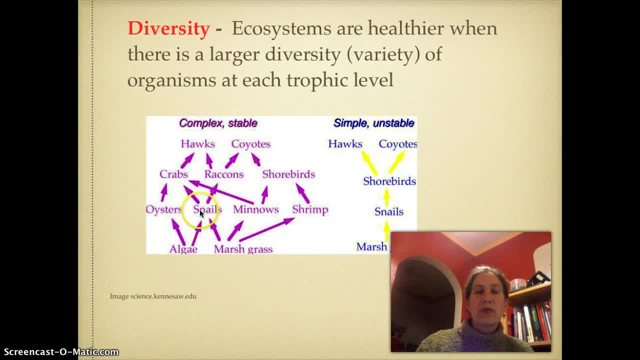 but through the marsh grass, And so it kind of allows kind of alternative pathways for the different organisms to get their needs met, Whereas you can see here, If there was a problem with the marsh grass, you know, pretty much everything kind of collapses. 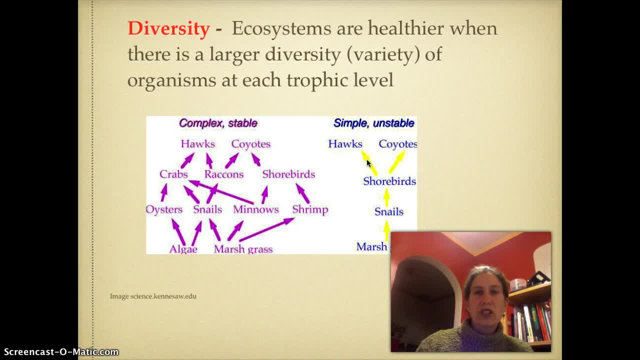 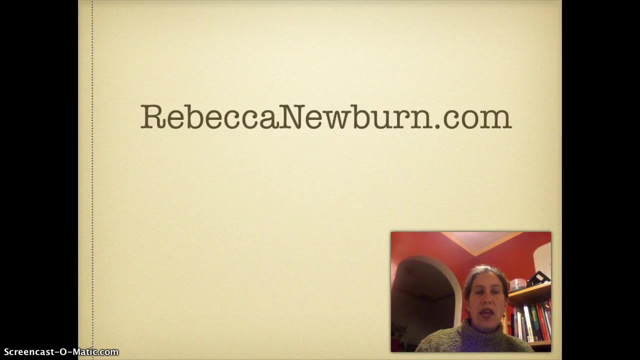 So simple systems are unstable. In our modern agriculture system, we have gone to a very simple and hence unstable system. So one of the reasons we're doing our food forest is to make a more complex and hence stable system. And, once again, if you need more information, you can go to RebeccaNewberncom and there. will be links for additional resources. Have a lovely day.